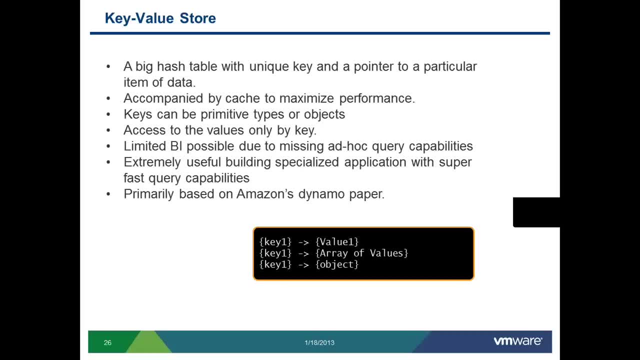 key and also the pointer to the item of the data. So sometimes they also get accompanied by a cache so that we can get a better performance. Keys can be primitive types or objects, So we can also have an object that is actually hashed into a key And then we can access. 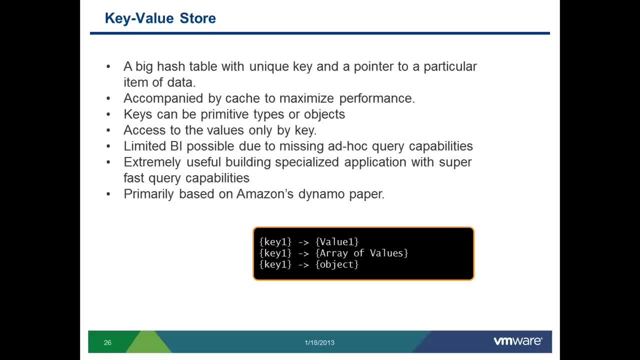 values only by key. So that is one of the fundamental behavior in a key value store. But of course some of the key value stores give some extra features wherein we will be able to even query by values, But the performance is a hit. 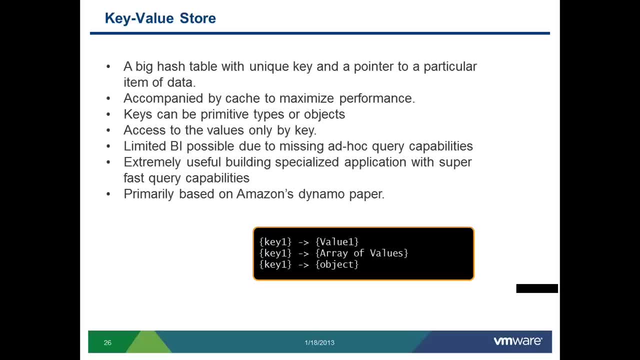 And because of this the amount of data that we can do with this kind of key value stores are typically limited And we can actually write specialized applications. that works only on top of the keys, So maybe we can go for a composite type of key where we will. 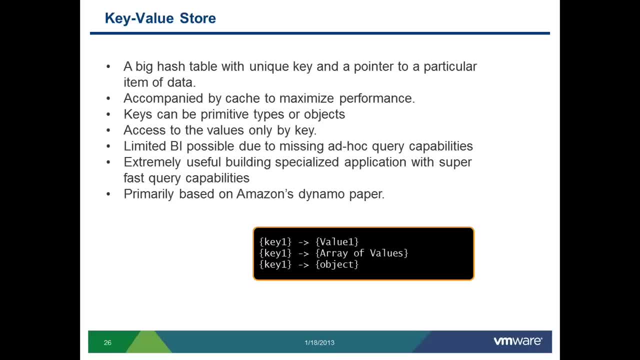 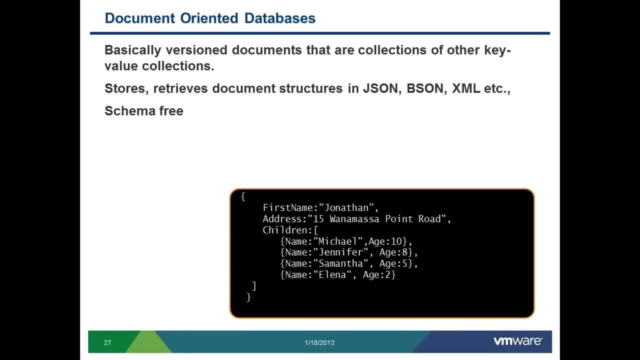 be able to do a bit of multi-dimensional analysis. But primarily they intended to create specialized applications And the initial philosophy came from Amazon's dynamo. So the next one is the document-oriented databases. So basically the documents are versioned documents. They will be stored against a key And also we can retrieve and store these documents. 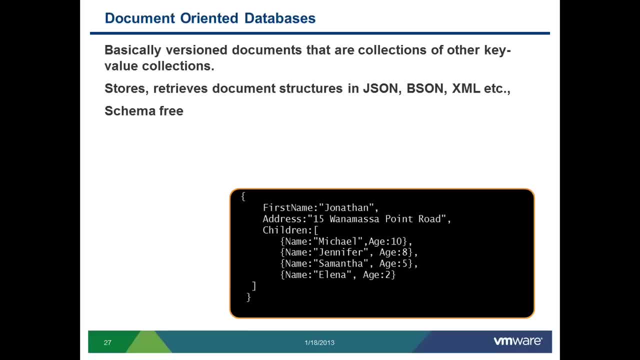 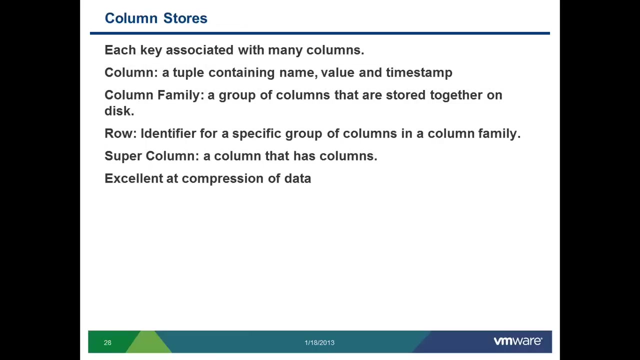 in multiple formats like JSON, vCM or XML documents. Sometimes NoSQL databases in fact classify the XML formats as XML documents. XML data NoSQL stores separately, But most of the NoSQL stores will support JSON And there's no, So the next one is the column stores, So each key is basically in this case associated with. 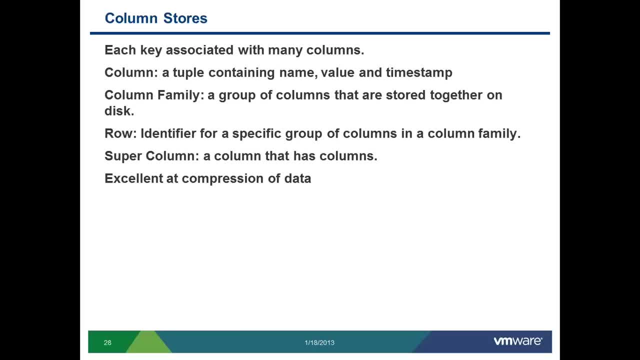 many columns. So a column is defined as a tuple that contains a name, value and a time stamp, And the column family is going to hear that it's a group of columns that are stored on a disk together So we can begin to write a column. But the reason why we did this is: 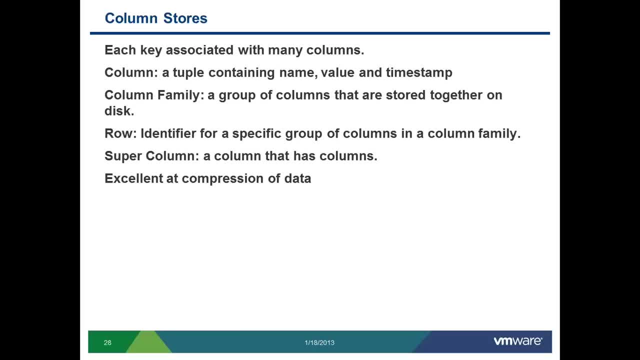 So if you are actually in the, if you are putting a column in the store, then we need to consider these aspects- whether the column belongs to a column family or not- And then row. basically it identifies a specific group of columns in a column family.